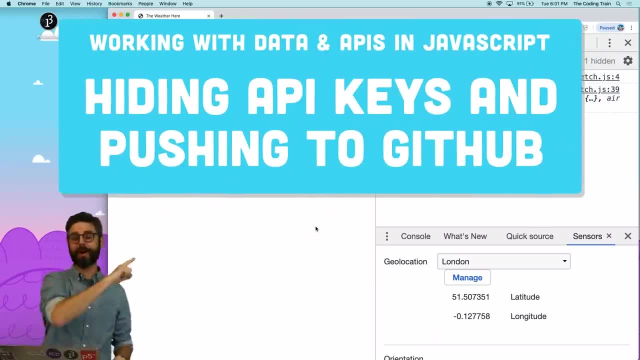 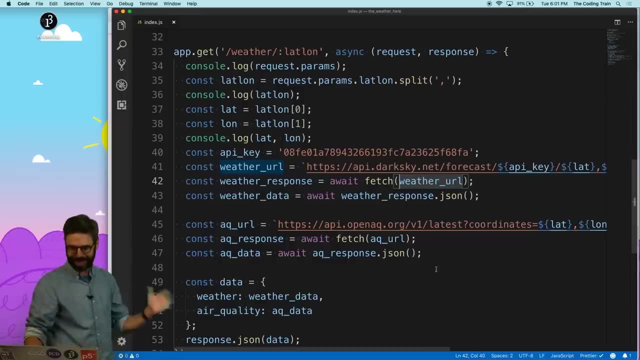 Hello, welcome to another Working with Data and APIs video, And in this video I'm continuing the Weather Here project And I just want to do one thing, one thing, a very important thing: I want to look at how to stop my API key from just sitting there. 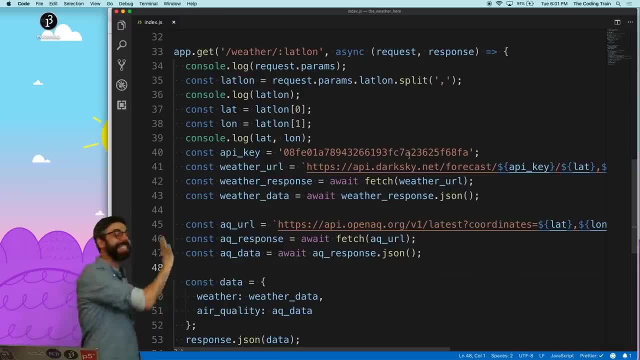 in my code. I mean, I have something a little bit better here which is at least the API key is in my server code, So no one could go view source just in the browser page and see API key is there. However, I would like to open source this: 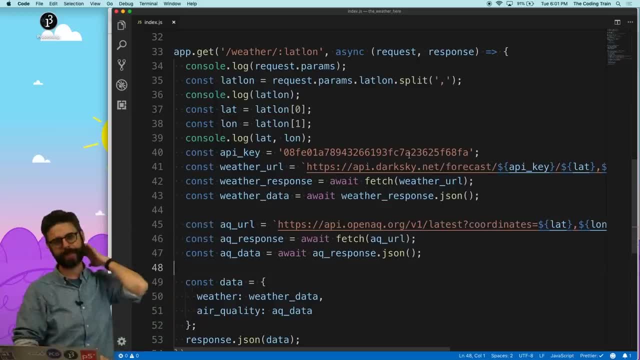 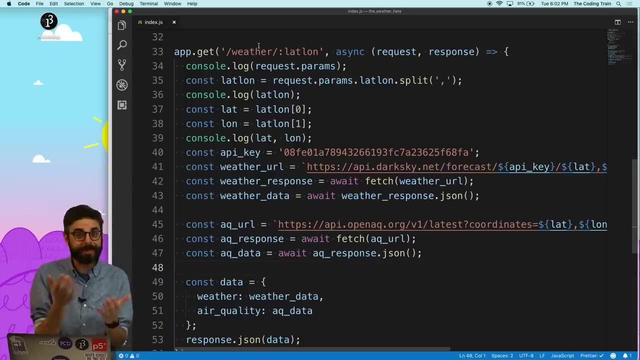 This is a public example I would like to post. I would like to share it. I don't want that API key just sitting there in the code, And the way that I'm going to address this is with something called an environment variable. An environment variable is a variable. 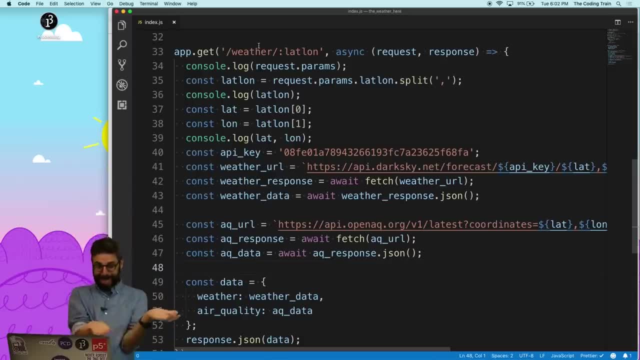 You know about variables. It's just like a thing I have in my code, like const API key equals. The thing is, I don't want my variable in the code, I want it stored in the environment. I want it to be something that's set within the operating system. 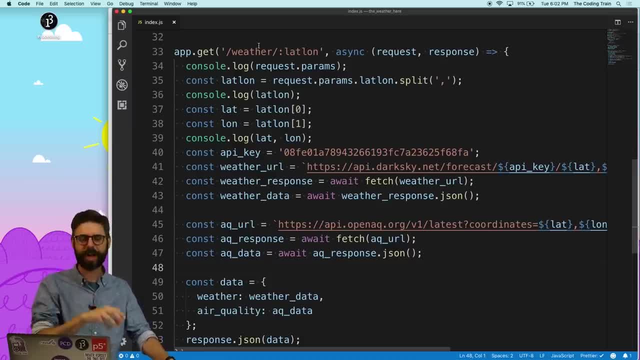 or whatever framework or system I'm using to run software itself and I'm just pulling it in the code. So how do I set environment variables with Node? Ultimately, there's no one way to do this. A lot of different platforms will have mechanisms for storing and retrieving environment. 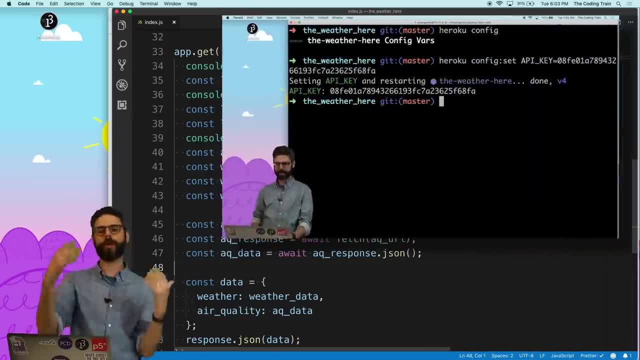 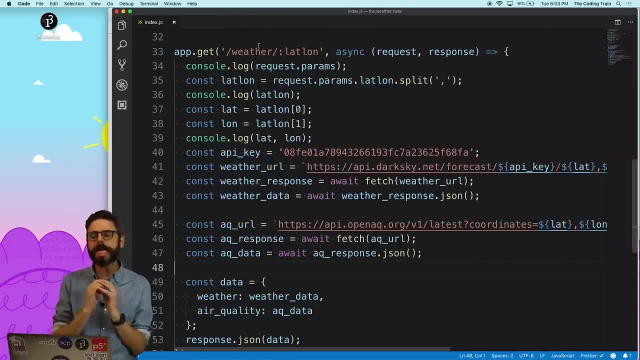 variables And in fact, when I look in the next video about deploying your project to a web server, we'll have to examine: well, how do I have environment variables saved on this particular web server? But a nice sort of clean way I could do it right here locally. 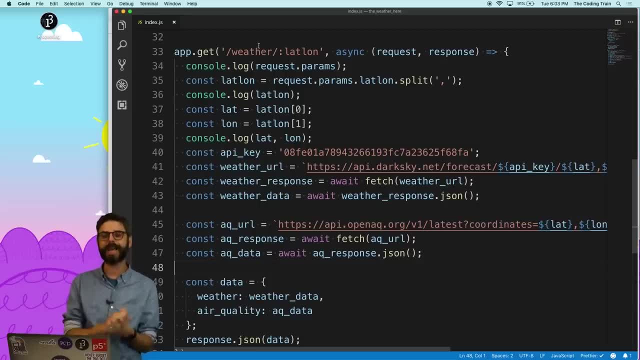 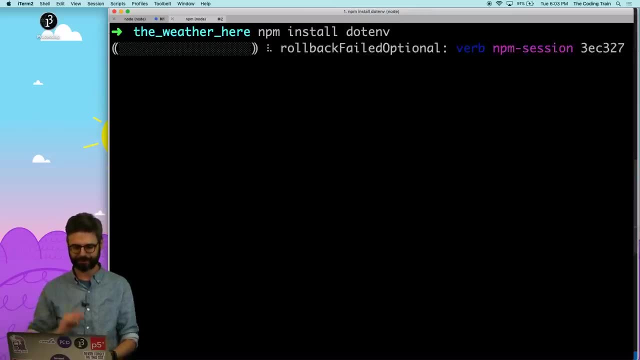 and demonstrate it is by using a Node package called env. So I'm going to go over to terminal and I'm going to say npm install And I'm going to say dot env. How env works is summed up perfectly in this one sentence. 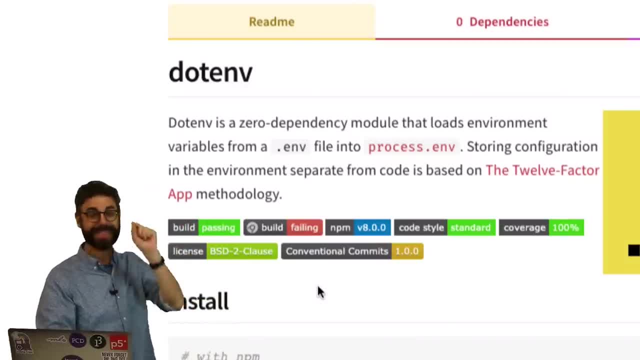 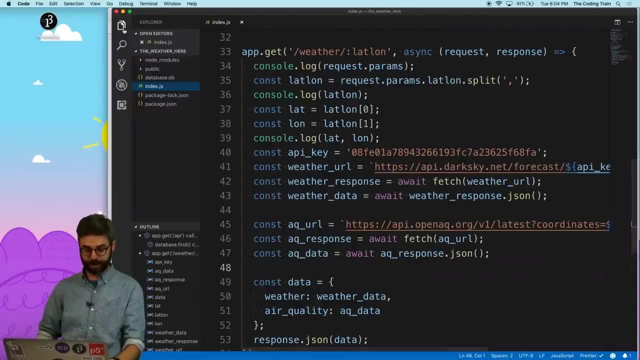 env is a zero dependency module that loads environment variables from a env file into processenv. Let me show you exactly what this means. I'm going to go over to the code. I'm going to just make sure I've got it here. 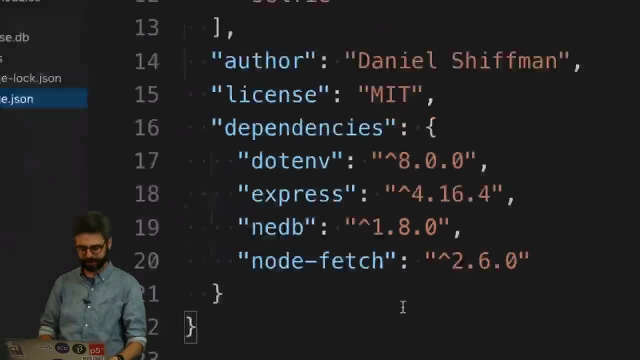 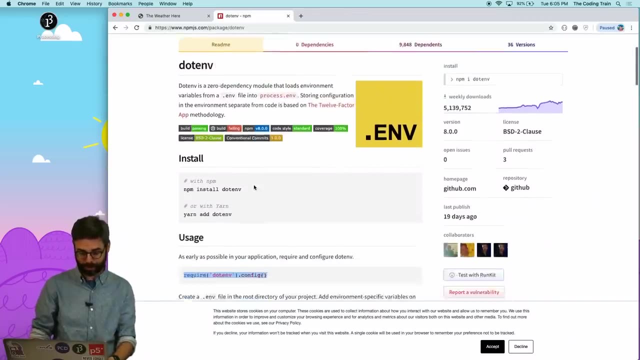 Yes, I've got the env package installed as a dependency. I'm going to go to my server code. In order for env to be in action, I need one line of code and it's right here. I want to say: require env and then call the config function. 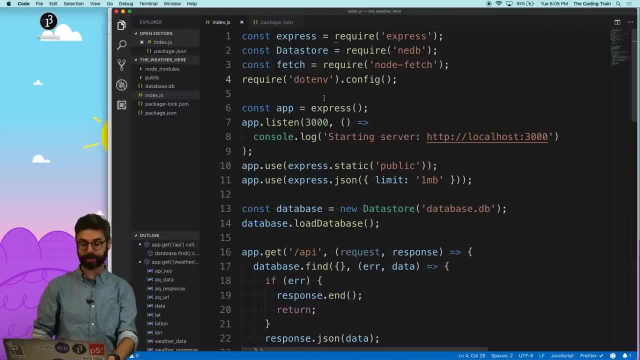 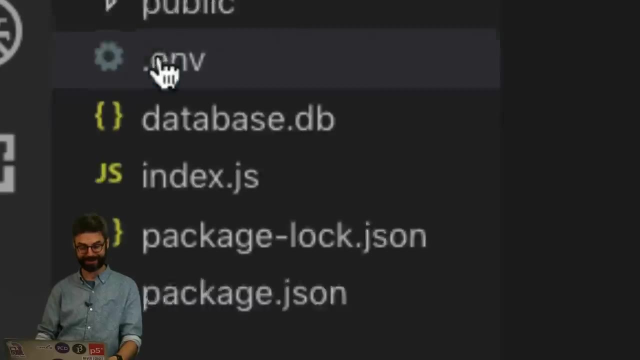 So this is going to tell this particular server to load anything that's in a file called env into an environment variable. So now what I need to do, in whatever text editor I'm using, is I need to make a new file And I'm going to call this file- guess what- env. 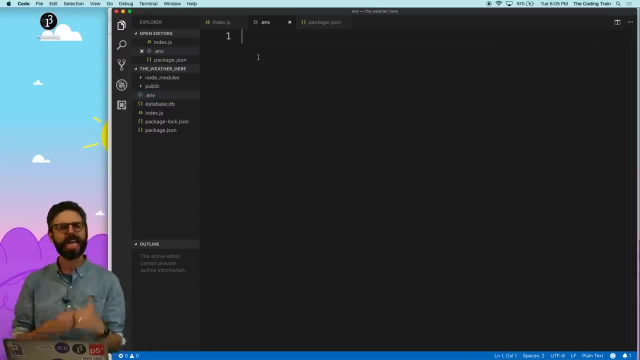 Then this is now a plain text file where I can put my environment variables. Typically, you might use all uppercase for an environment variable, Although I don't know if that's necessarily required. But I'm going to say API key. API underscore key equals. 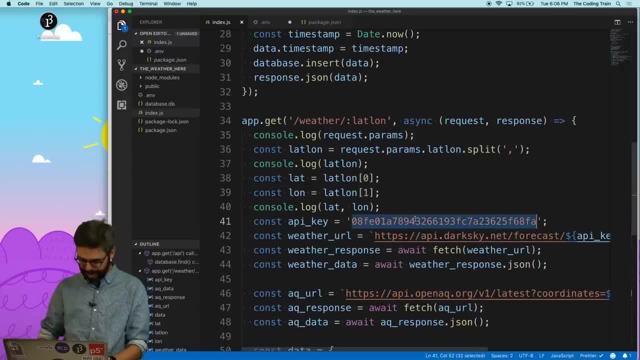 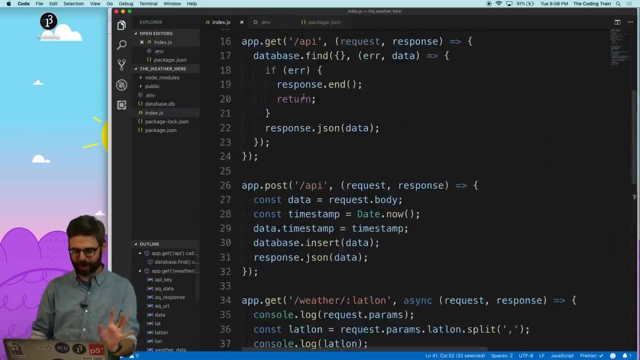 I'm going to go back to my code, I'm going to grab the API key, I'm going to go back to env and I'm going to paste it in. So now I just want to do one thing now in the server. 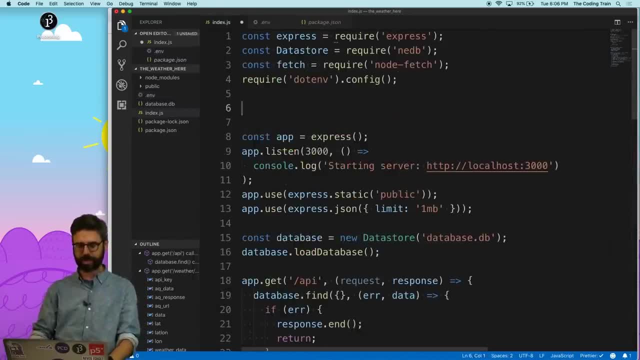 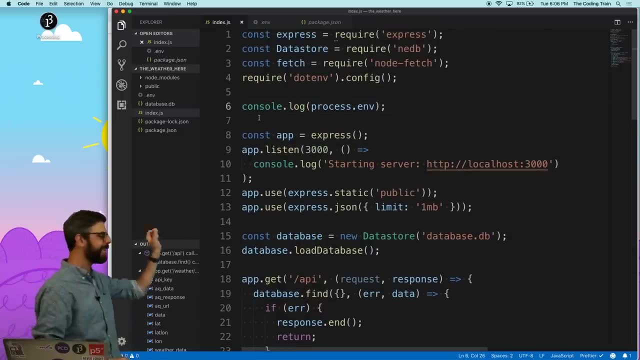 I want to log consolelog processenv, And we should see that anything that's in the env file, as long as I call requiredenv, a call config will now be inside of processenv. So let's restart the server. 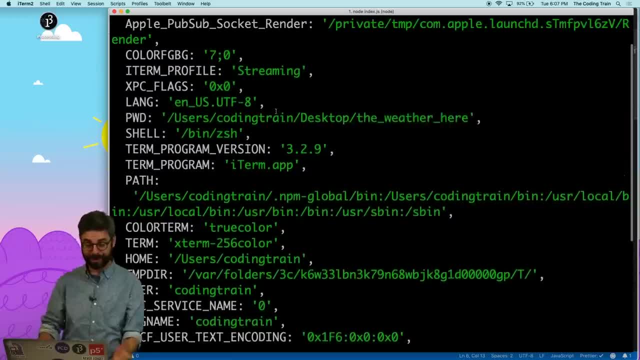 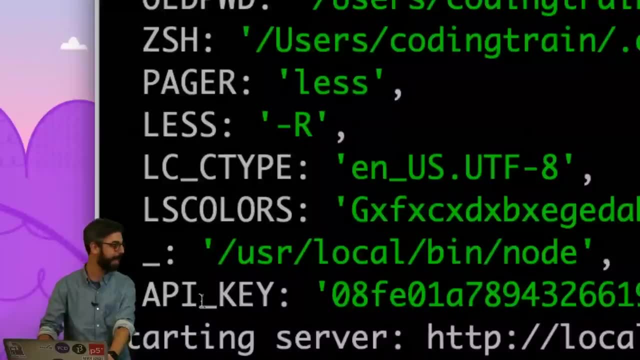 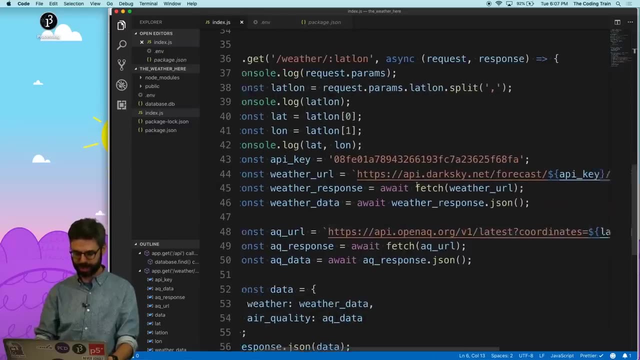 And we can see: oh boy, whoa, a lot of stuff. Look, there are lots of environment variables already there, But look at this: I've added one right here at the bottom, API key. There it is, which means I can now go here into my code. 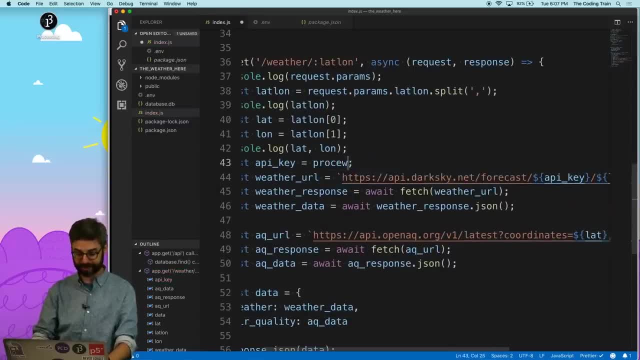 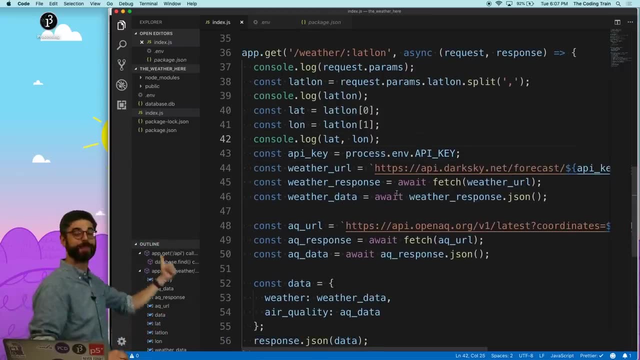 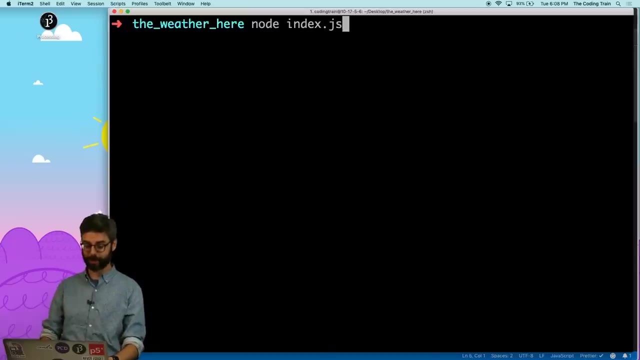 And I can change this to be: API key equals process EnvAPI underscore key, So I can pull this API key from the environment variable. It's no longer in the code whatsoever. Let's remove that console log. Let's make sure the application is still working. 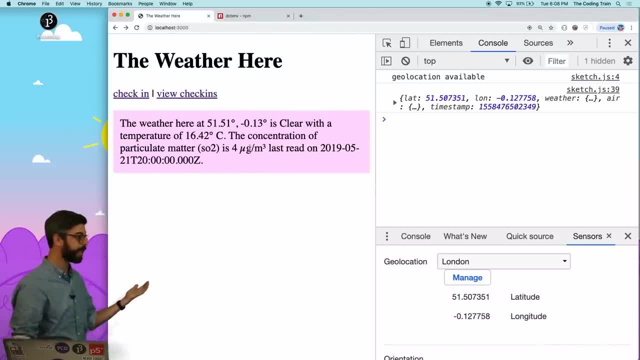 I'm going to run the server, I'm going to hit Refresh And it looks like I'm still getting the weather information When I go. look at the check-ins: everything is still there. I check in and I'm still getting the weather information again. 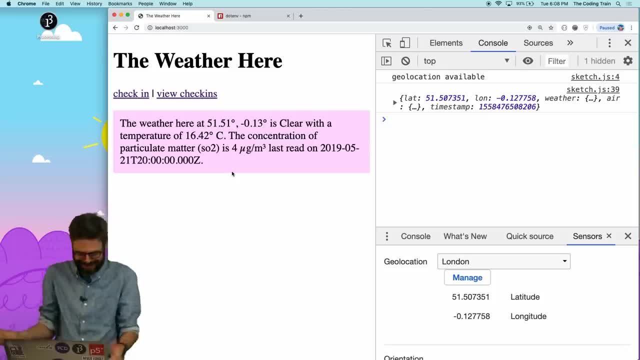 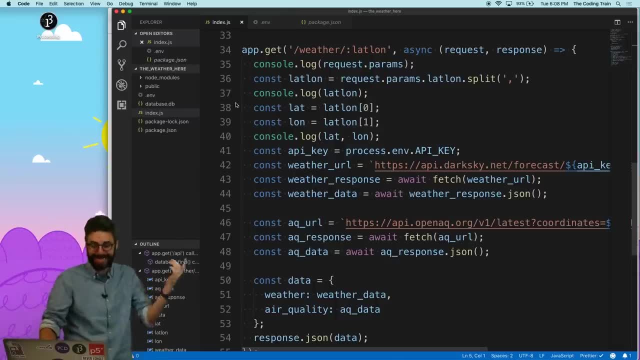 But oh, oh, you might be asking: how is this any better? Sure, there's no API key here in the code. It just says processenvAPI key. But you have a file right over here that has the API key in it, right there. 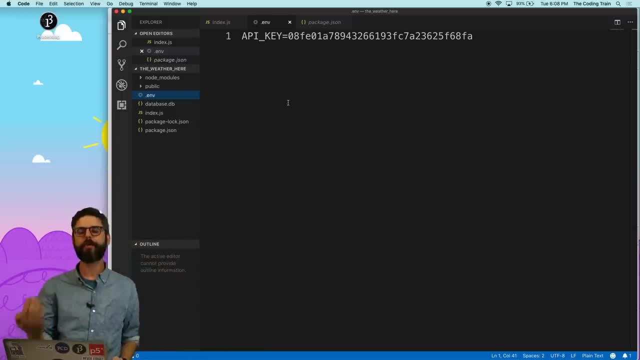 And so this is a convention. So it is a convention for environment variables to be stored either in an env file or through some other mechanism, based on whatever server you're using, but not to be published when the code is published. So this begs the question. 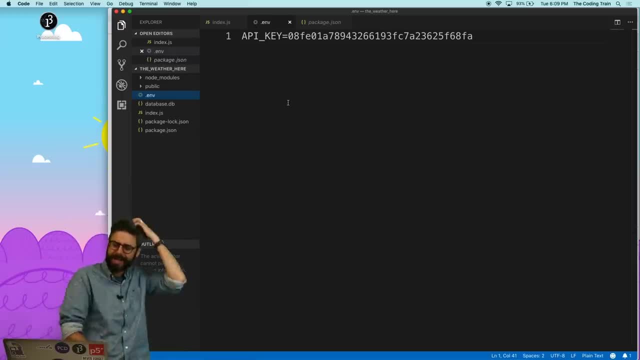 Am I bothering to publish this code? Is this fine? How do I? what do I do when I deploy this? So to some extent, this is really going to matter when it comes time to deploy this project to a web server somewhere- And I'm going to do that in the next video. 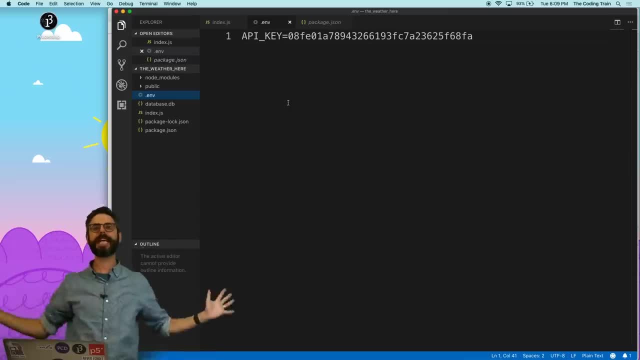 And we'll have to revisit this environment variable question here. But let's just say I just want to publish this as an open source project on GitHub, So why not a little extra feature in this video? This feature is also about hiding your API keys. 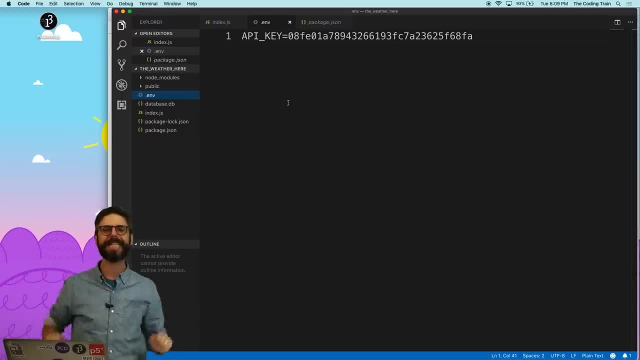 and then publishing your project onto GitHub, And I'm going to do it in the most lightweight, simple way possible. Now you might be asking yourself: what's GitHub, What's Git? Those could be completely unfamiliar things to you, And so I'm going to refer you in the video's description. 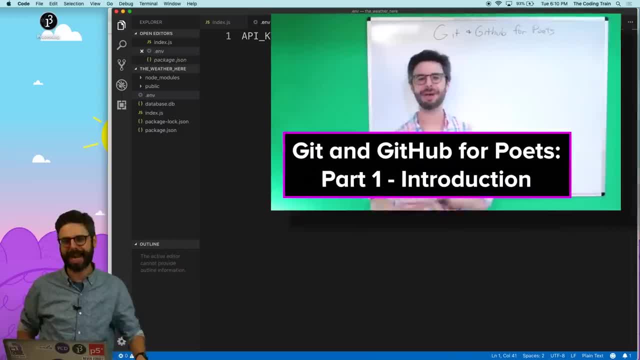 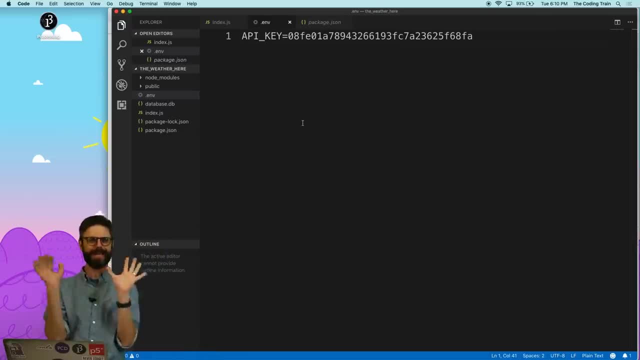 to some additional information about that as well as some video tutorials that I've made of the basic introduction to Git and GitHub. So this won't be comprehensive at all. I'm going to kind of assume some knowledge but try to be as beginner friendly to you. 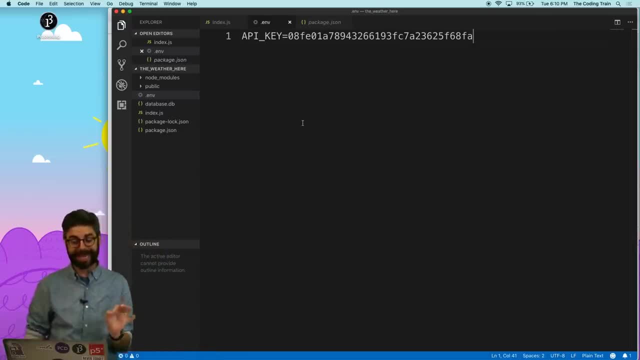 as possible, too, when walking you through the steps. So the first thing that I want to do is actually create another file. I'm actually going to create two other files. I'm going to make a file. I'm going to call it env. 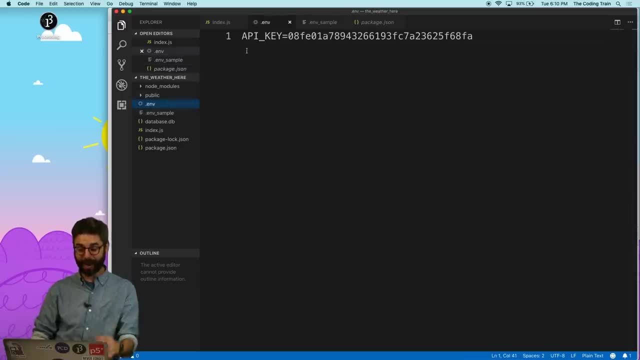 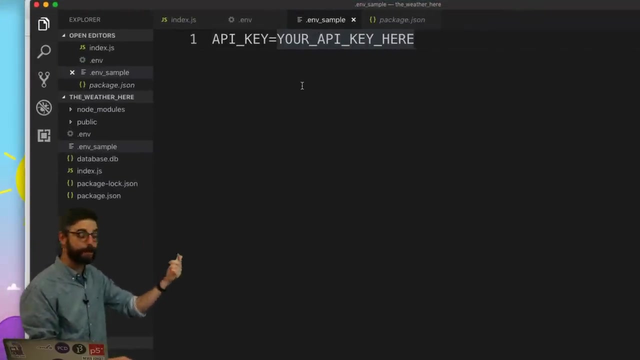 I'll call it like sample, Because I actually want, when I publish this, to publish a file that tells you how to put your API key in, And so I'm just going to say your API key here. So this env sample file is the sort of sample. 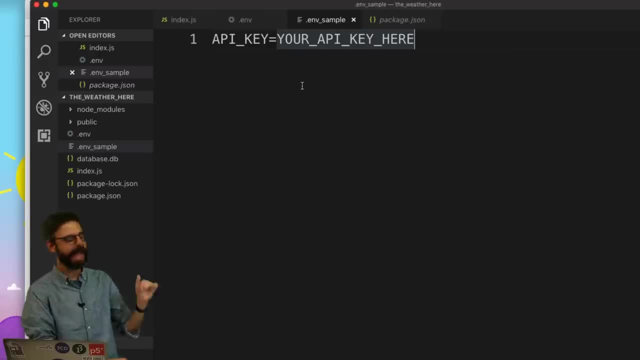 It's sort of implying: rename this file to env and put your real API key in. OK, So I'm going to put my API key in here And I could probably in a read me or somewhere. I would want to provide more context and information. 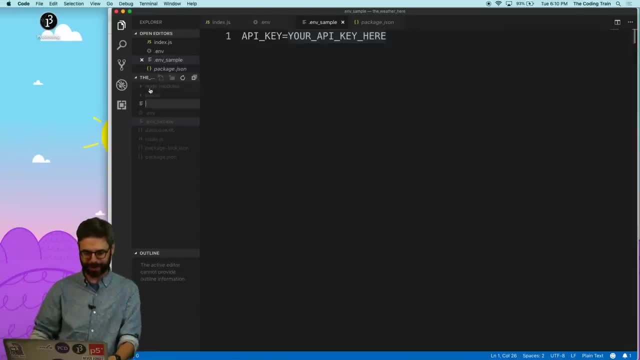 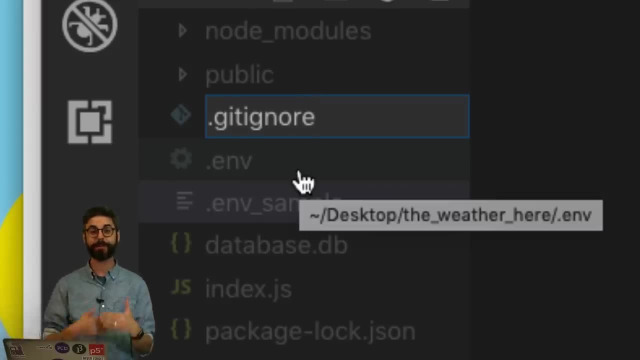 But this is a nice starting point. Then I need yet another file. I'm going to create another file and I'm going to call this gitignore. So this is really important. Git is version control software that keeps track of all of your files and various versions of them. 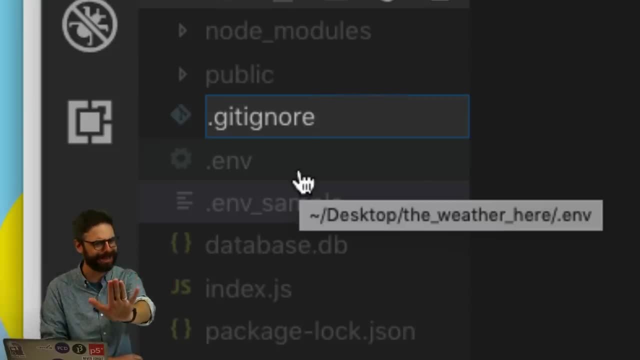 What gitignore does. it says: hey, hey, hey, hey, don't keep track of this file. This is my own personal secret stuff. I just have it here on my machine. Don't keep track of it with Git, Don't upload it anywhere. 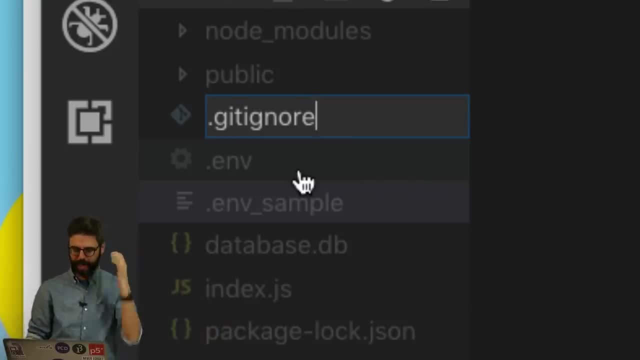 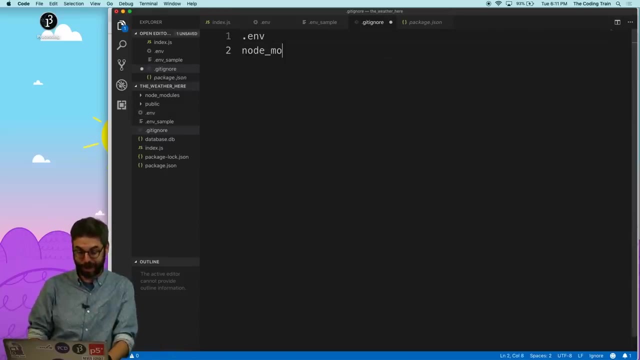 Don't ever use it anywhere. So in order to do that, so I'm going to create that file. And what's the file I want to ignore? I want to ignore env. I actually also want to ignore some other stuff like node modules. 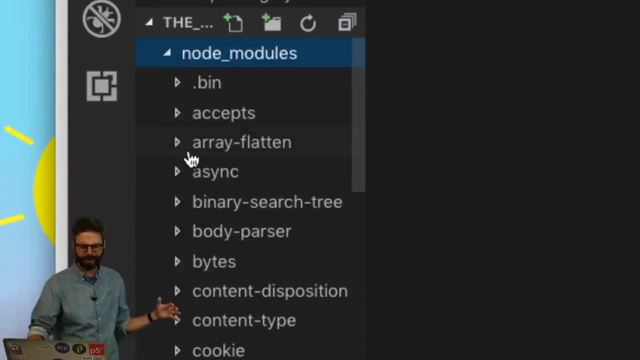 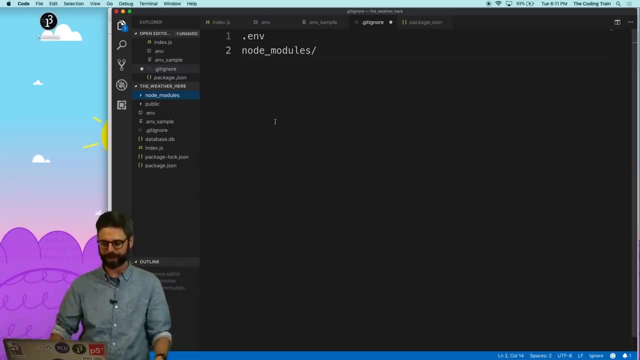 I don't want that node modules directory. This is all of the other people's code, of all these packages. It's a huge amount of stuff. That's not something that I want to publish and upload when I'm publishing a project, But everything else I could presumably 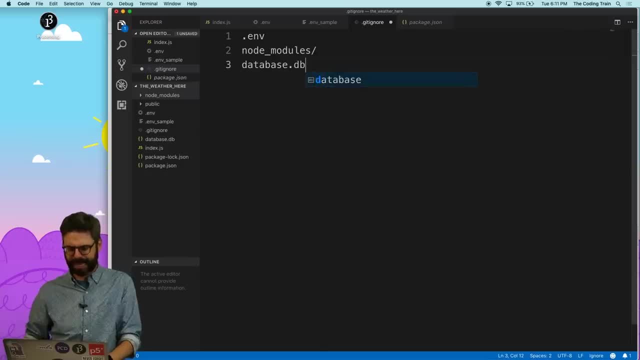 maybe ignore the database. Maybe I don't want to keep the database, but I don't really care about that right now. So I'm just going to, I'm going to leave that be. I kind of want to ignore it. Let's ignore it. 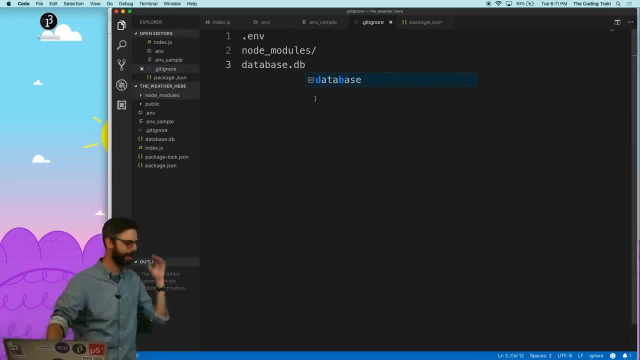 This is an interesting question. I'm not so sure whether it makes sense to ignore it or not, but I'm going to ignore it. The next step that I need to do is go back to terminal. I'm going to go back to terminal. 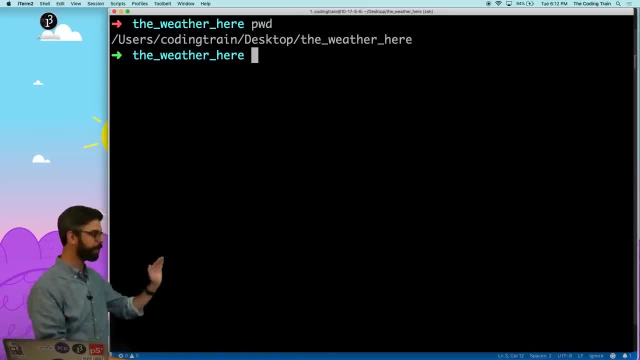 I'm going to quit the server. I am here in the directory of this project- the weather here- And I'm going to type the commands. git init: That's going to initialize this folder as a Git repository. Git init: So it initialized an empty Git repository. 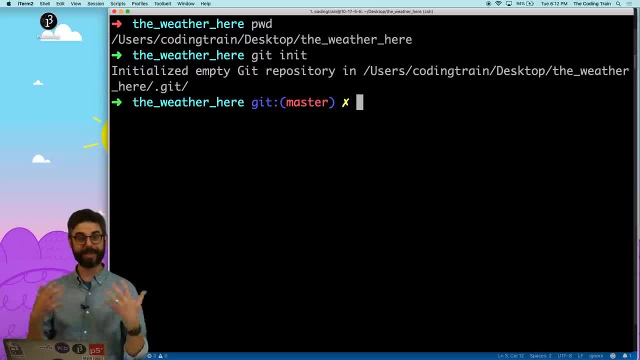 Then I'm going to do my first commit of everything that's in the directory. A git commit is a moment in time saying, hey, this is a particular set of changes that I want to snapshot as a moment in time with this project and save for its history. 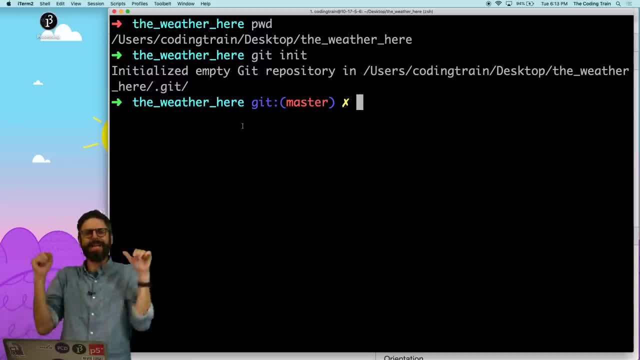 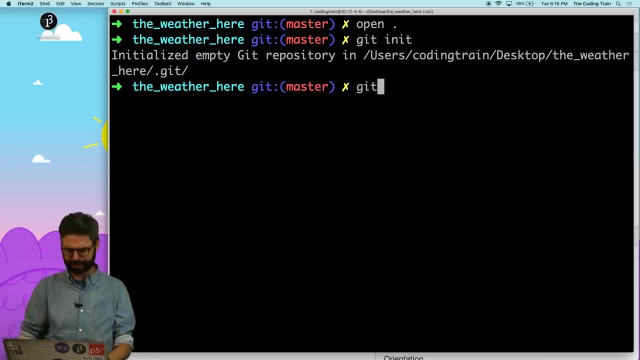 And the truth of the matter is this is my first commit, So I'm just really saying, hey, can you add all this stuff and save it? So to do that first commit, I'm going to do this in two steps. I'm first going to say git add, which is, add all these new files. 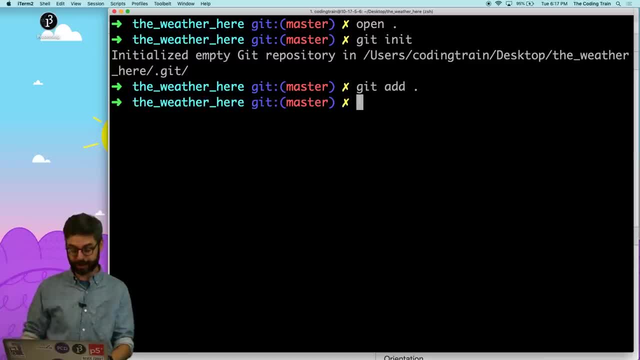 Git add, and the dot means add everything. Now I'm ready to type git commit. Now you might think this is a little bit strange. Why is it two steps: Git add and then git commit, Don't I just want to commit all the stuff? 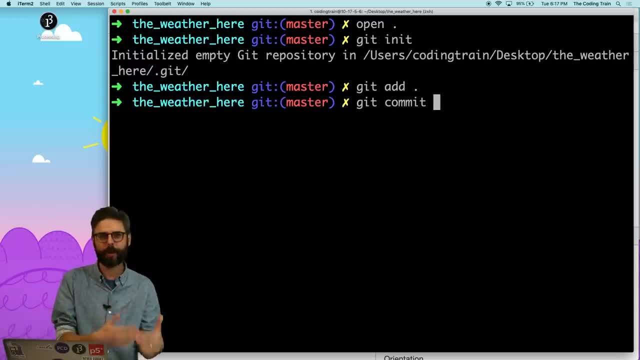 Well, this has to do with how Git works as a software system. There's a staging area that files get added to. Then those files can be committed and things can be moved around in all sorts of complex ways, And this is something that I cover in more depth. 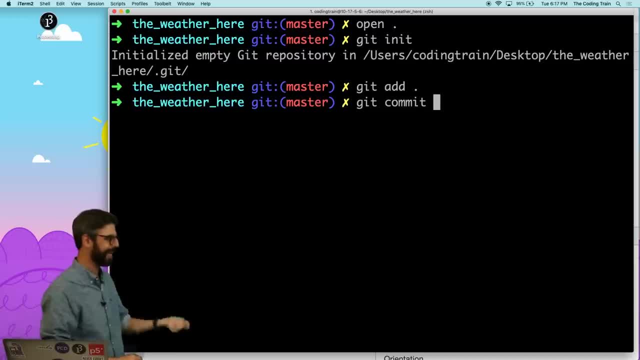 in that other Git and GitHub video series. But for now, all I want to tell you is that I need to add all the files and then I want to commit these files. So I'm going to say dash m and I'm going to put a little message here. 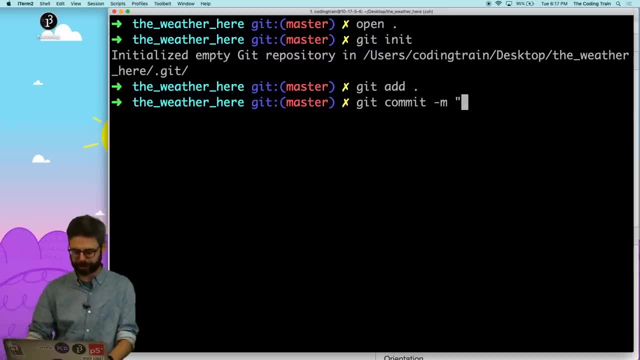 There's more ways that you can write longer, more thoughtful messages, but I'm just going to say this is the code from whether here. as of video, I think this is going to be video 5-4.. And I'm going to hit Enter. 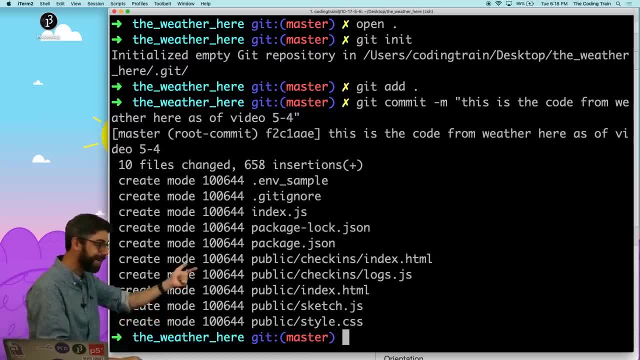 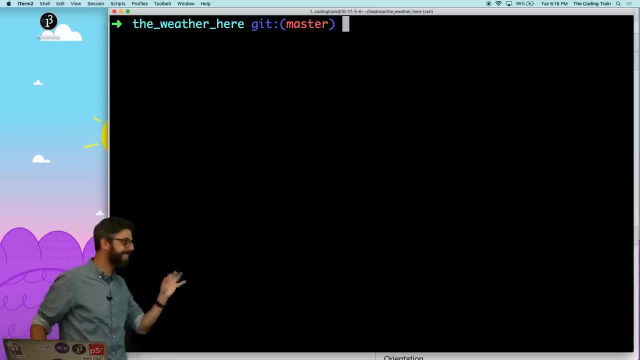 And then all this stuff has been added. Now look, if you look at this list, do you see node modules there? Do you see dot env there? No, because those were ignored with git ignore. The next thing that I want to do is put this on GitHub. 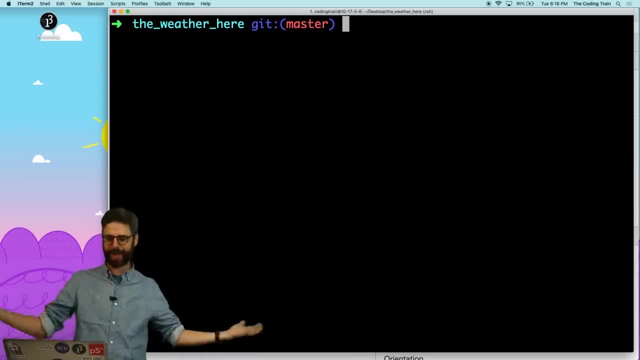 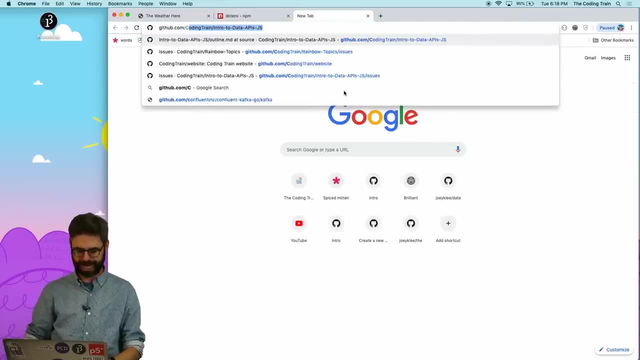 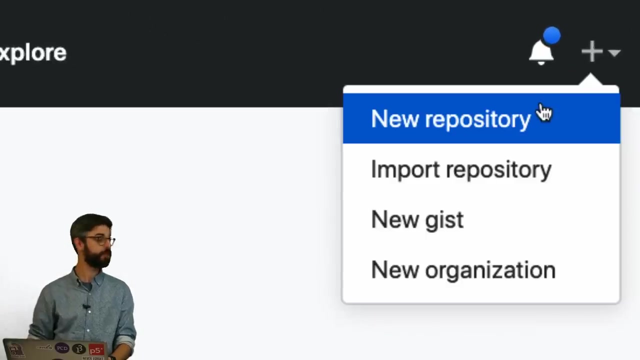 So GitHub is a website that can host your Git repositories. This is now a Git repository sitting on this laptop, So I'm going to navigate over to GitHub slash Coding Train. I'm going to come up over here. I'm going to click this button to create a new repository. 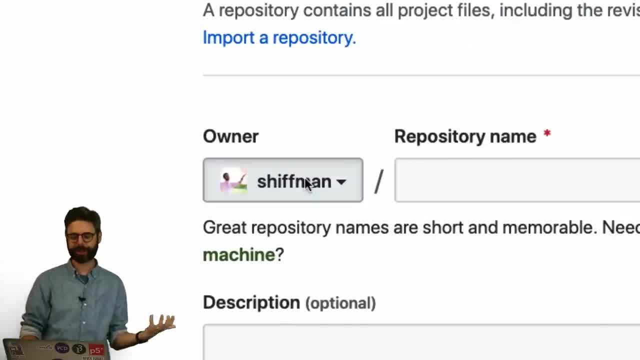 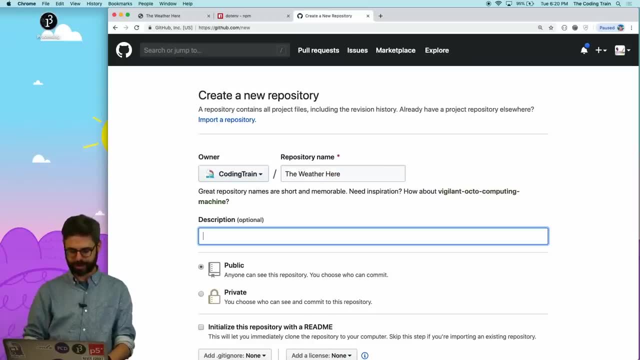 Then I want to go here and I want to make this. I have a GitHub organization which is called Coding Train, So I'm going to select that and then I'm going to make a project called The Weather Here. This is based on Joey Lee's project The Weather. 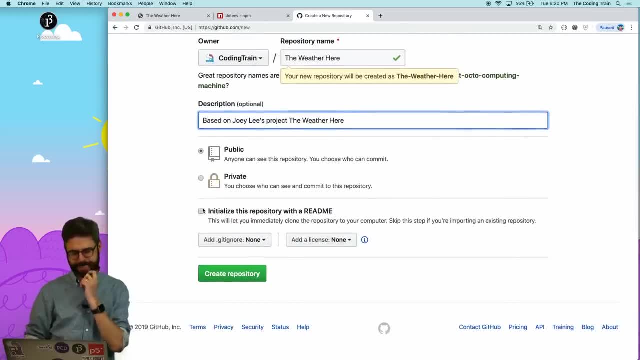 The Weather Here. I'm going to initialize this with a readme: No, There's so many different ways to do all this stuff And I think I show you in other videos different ways, But what I've actually, the steps that I'm following here. 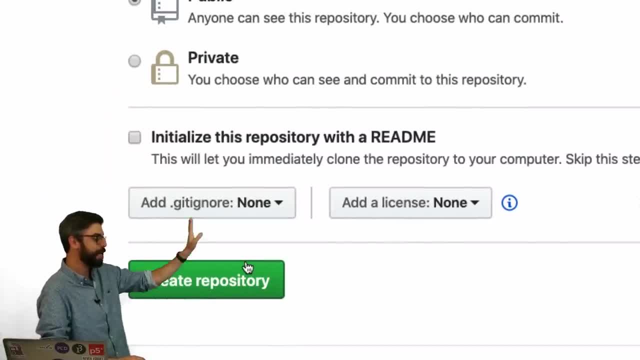 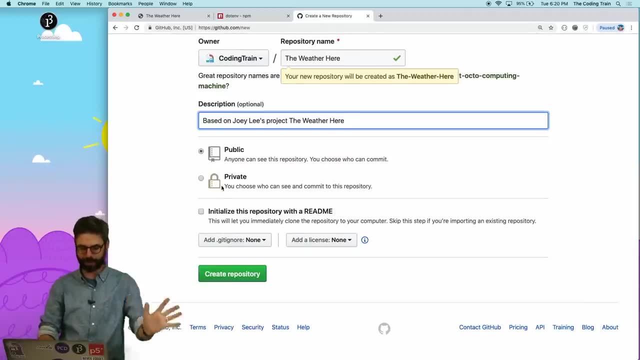 I already created the Git repository, So I don't want to make a new one. I want to just up. I just want to sync the two. So I'm just going to click: now I want this to be public. I'm just going to click Create Repository. 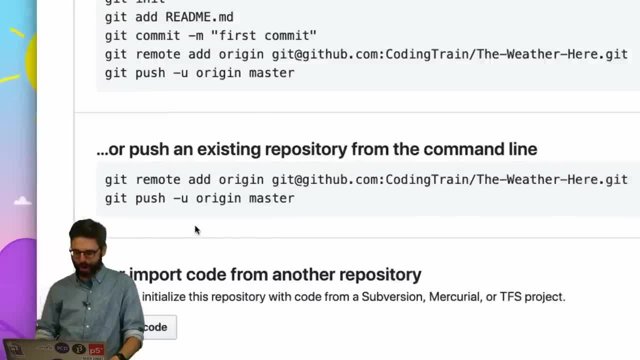 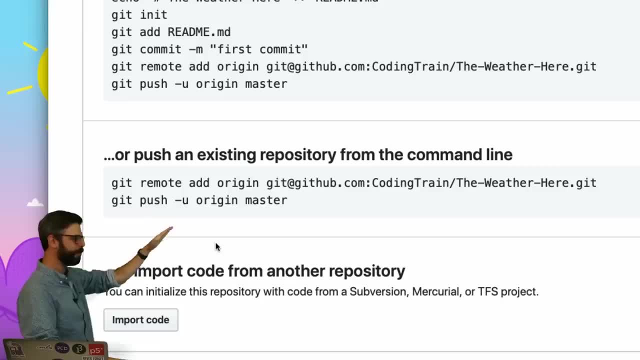 And GitHub is so nice to me. It's just saying, oh, this is all I need to do here. All I need to do is add this as a remote, the Coding Train Weather Here. add as a remote And then I can push, which means send it. 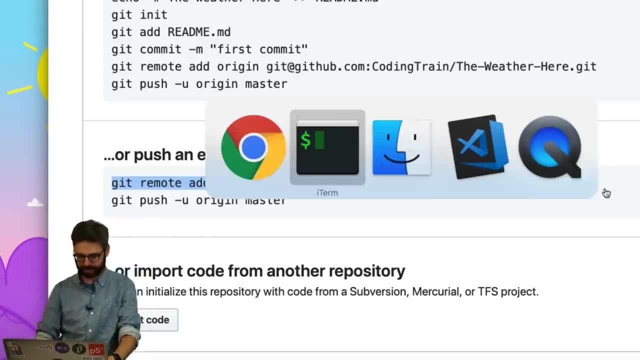 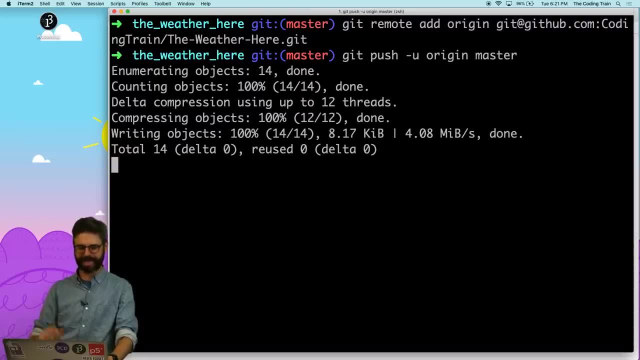 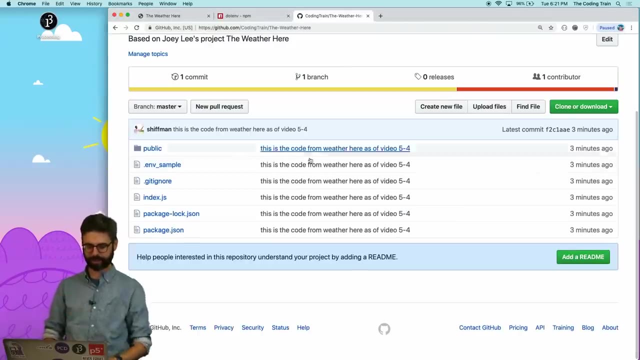 So I can just literally copy paste to this command, go back to terminal, type that in and copy this command, go back to terminal, paste that in, And I have sent all of the code to GitHub. I hit refresh here. This is the full project. 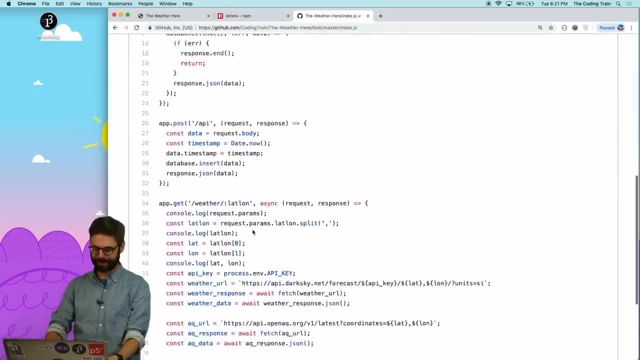 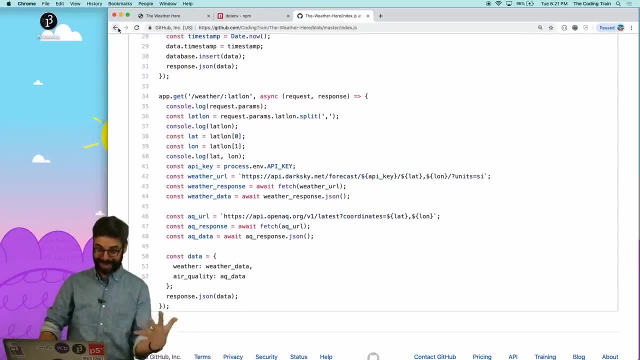 And if I navigate in and look at indexjs, we can see that the code- oh, I mean, sorry, the API key- is come from the environment variable. But the environment variable is not set. There's just an environment sample which is showing how to add your API key.